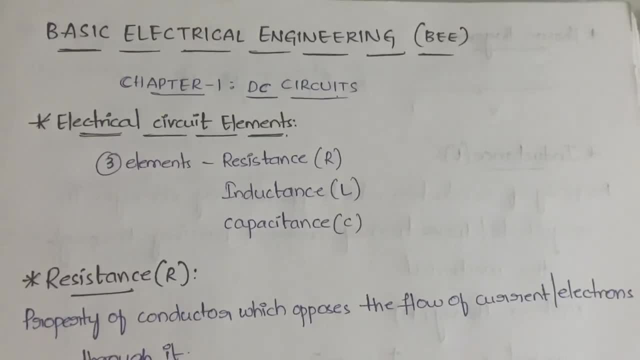 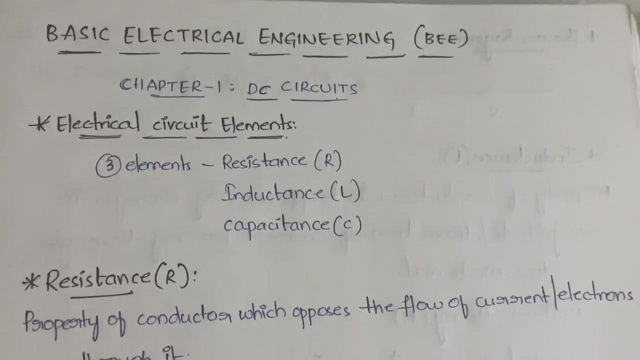 So I used to have this subject in my second year, first semester. So when I have the subject I was like why, why, why do we have the subject and why they have included this for CSE students? So I did not like so much but still, you know we have to, since they have included, we have to clear. but it was some a bit difficulty to many of my friends. 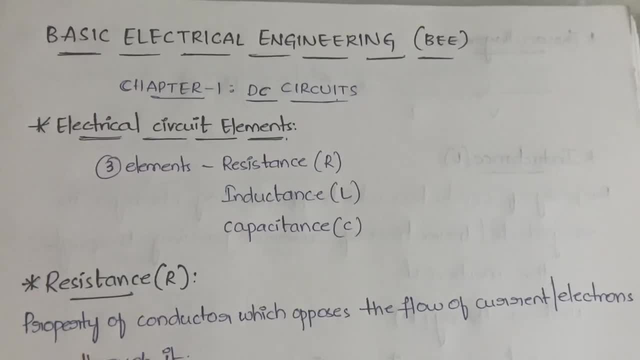 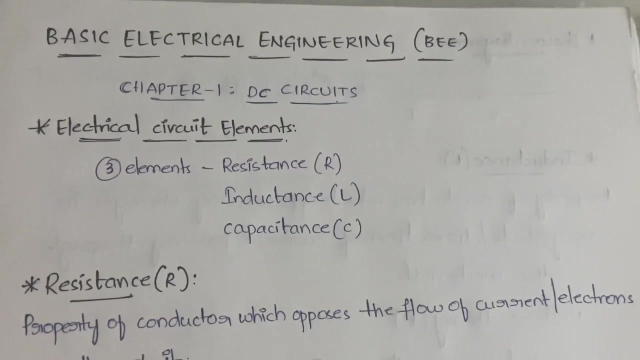 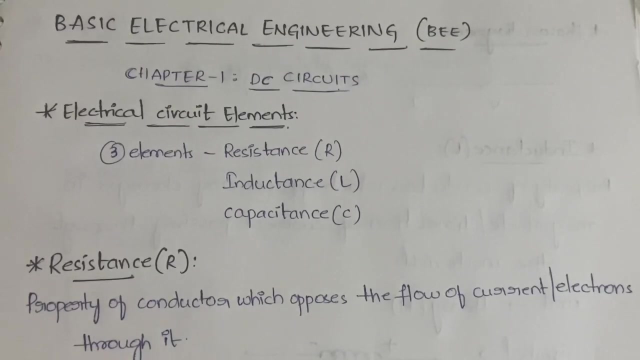 So, and even so many out, also outside also so many people will say: BW is hard, BEEE is hard. So that is why I am here. So that is why I am here, So that is why I just want to make it easier for you. I will try to simplify it for you in my own way and make sure that you will be writing well in the exam. Okay, So in this video, chapter one, which is DC circuits, we are going to learn basic electrical circuit elements. So we have three elements. So what are those three elements we will be learning in this video? So those three elements are: first of all, you know what is DC? right? DC, AC. DC is nothing but DC. 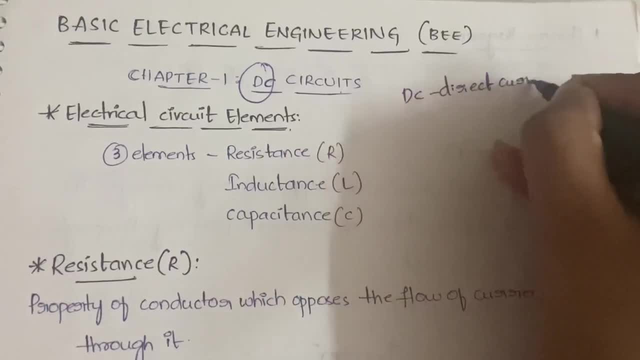 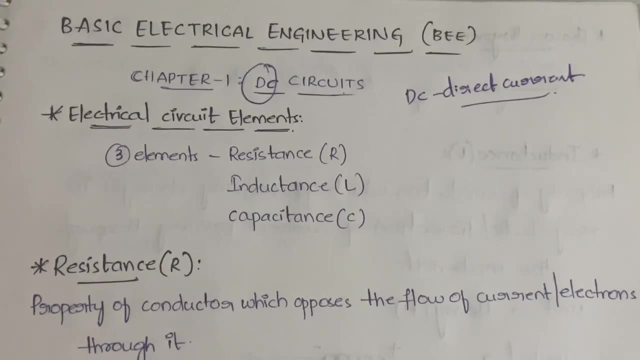 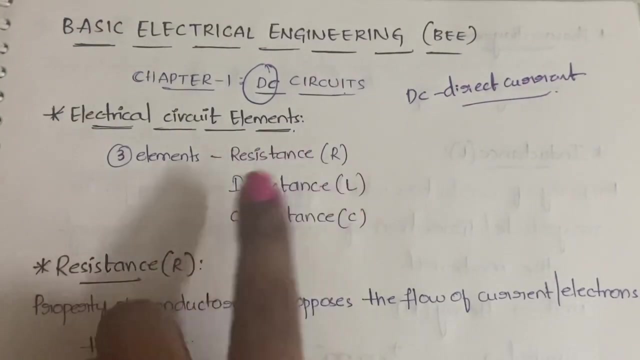 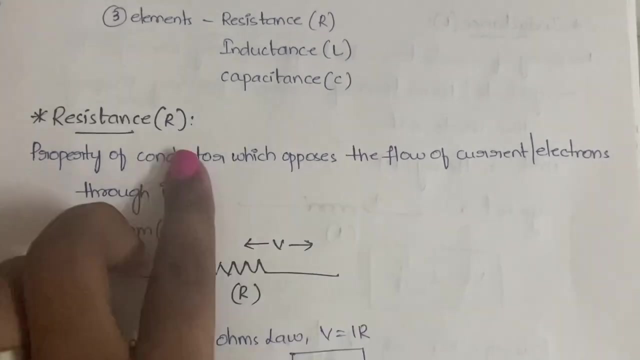 Direct current. AC means alternating current, So DC is direct current And in this we have three elements, three circuit elements. we are having resistance, inductance, capacitance. Resistance is denoted by R, inductance by L and capacitance by C. Okay, Now let us see about each of them. First, resistance: Resistance is nothing, but it is a property of a conductor. or you can take any material also, but that has to be a conductor. 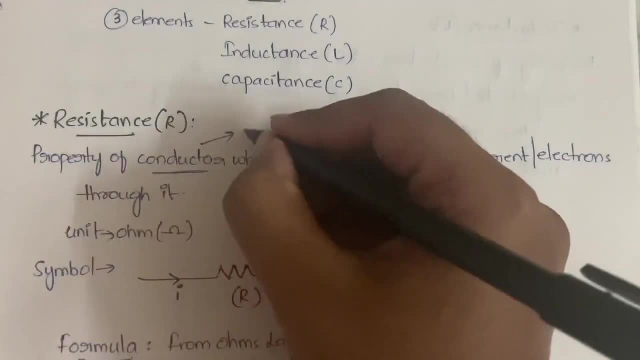 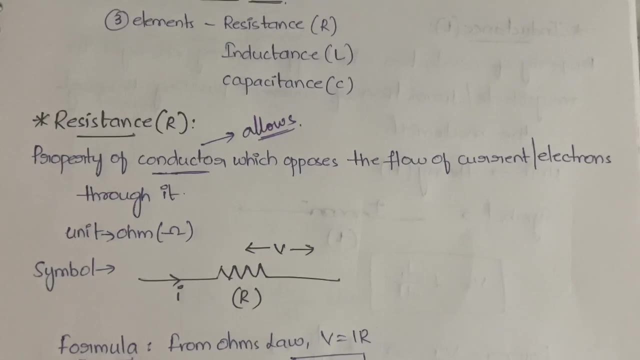 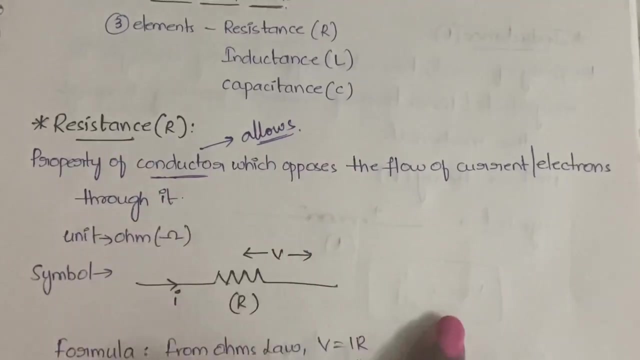 What do you mean by a conductor? Anything which allows the passage of electricity. You know: conductor, semiconductors, insulators. right Insulator will not at all allow electricity, Semiconductors will partially allow, and conductors, they will allow the passage of the electricity through them. Okay, So it is nothing. but it is a property of a conductor which opposes the flow of current or electrons through it. See, in some books I have seen it as current, In some books I have seen it as electrons. So 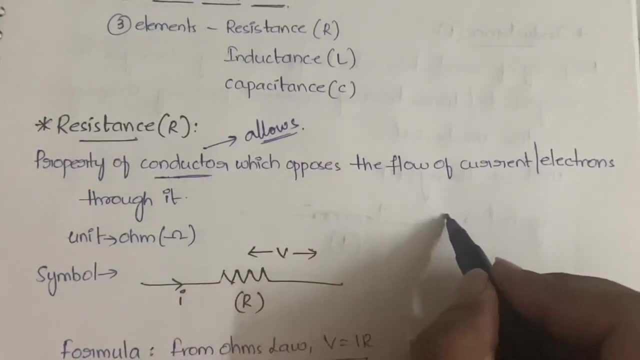 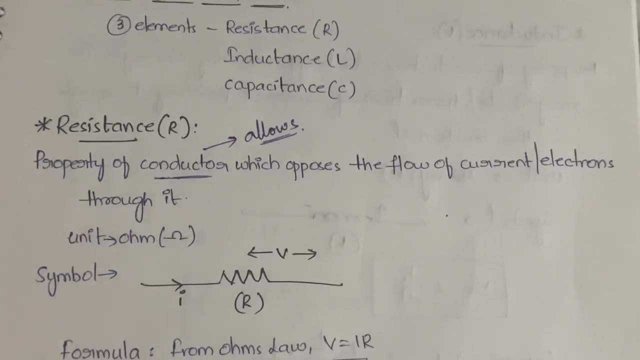 simply, when a current is passing in a conductor, okay, the flow of that current or electrons will be opposed with the help of a resistance. Okay, So usually resistance. this is a symbol before symbol unit. The unit of resistance is ohms and it is denoted in this way And the symbol is: we will be having, like this, speed breakers. Okay, So this is resistance and the current V is nothing but the potential difference. Okay, 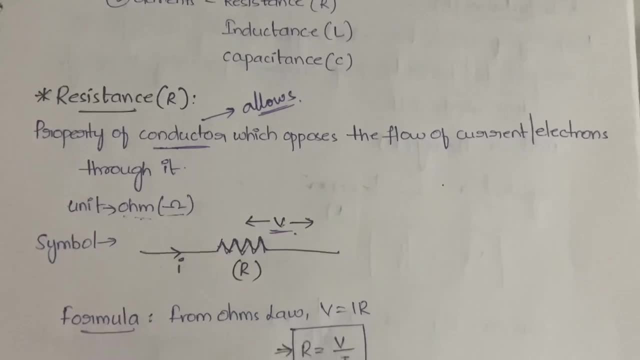 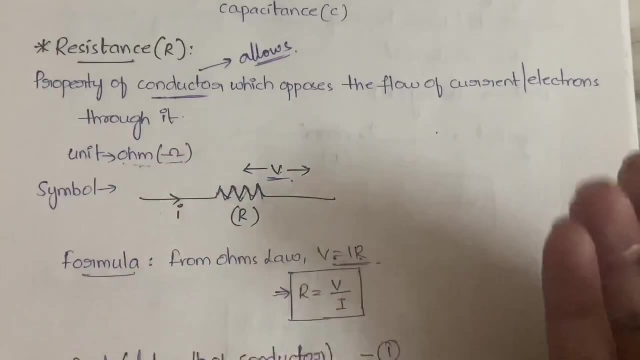 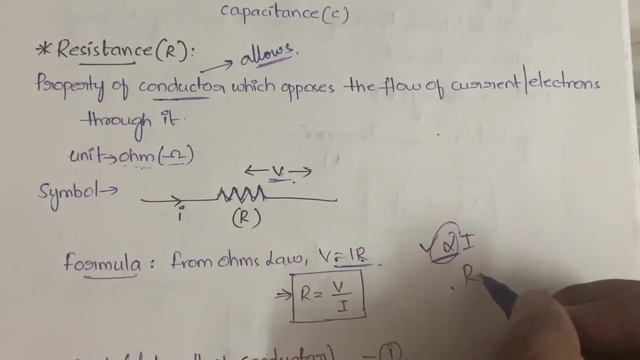 Next, what is the formula to calculate the resistance? then You know from Ohm's law: V is equal to IR. So what is Ohm's law? I will explain you Basically. Ohm's law is nothing but potential difference across the conductor will be directly proportional to the current flowing through it, And when you remove this proportionality you will be getting the constant, which is nothing but the resistance. Okay, So about Ohm's law and about the working problems. 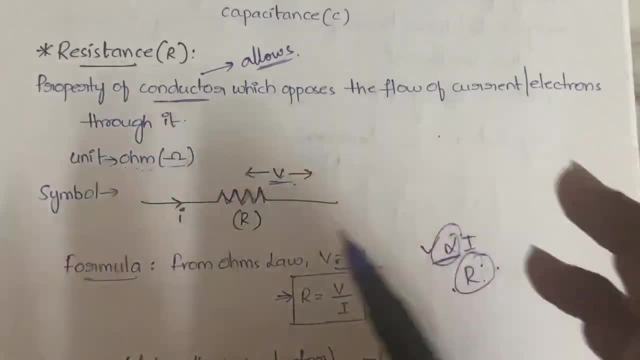 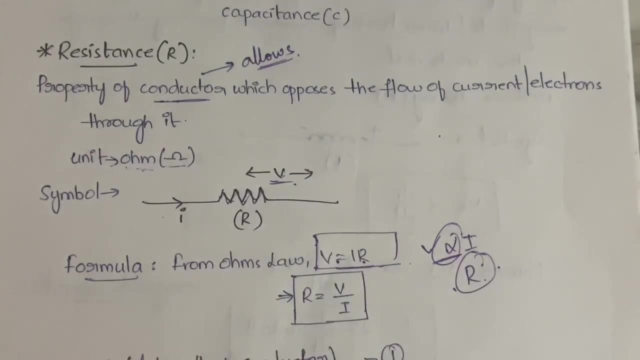 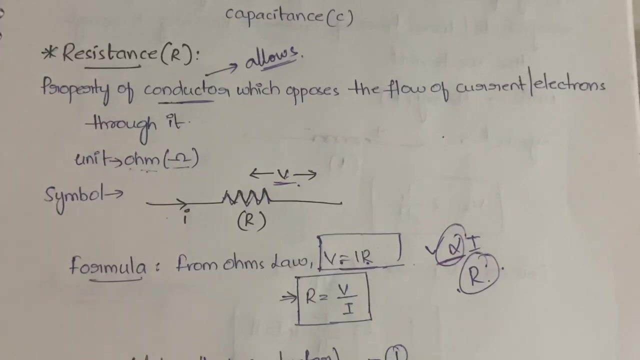 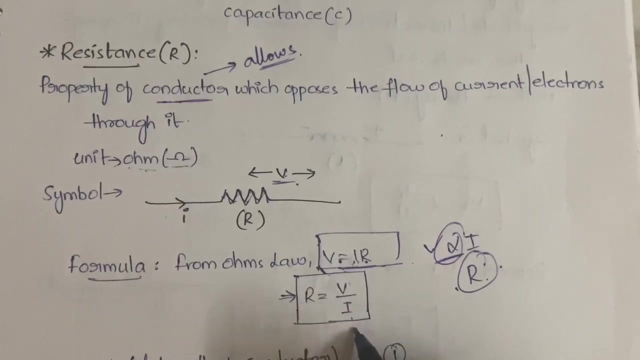 some example problems of Ohm's law. I will do it separately, But for time being you just remember Ohm's law is nothing, but V is equal to IR. You already learned about in your engineering in your 10th grade. also For me in Narayana, I guess I learned it in 7th or 8th grade. I don't even know what is conductor, what is resistance- nothing I know in that age. But okay. So when you send this I over to this side, it becomes divided by, and R is equal to V by I. Okay, And we also have another formula. So when you are taking a conductor, 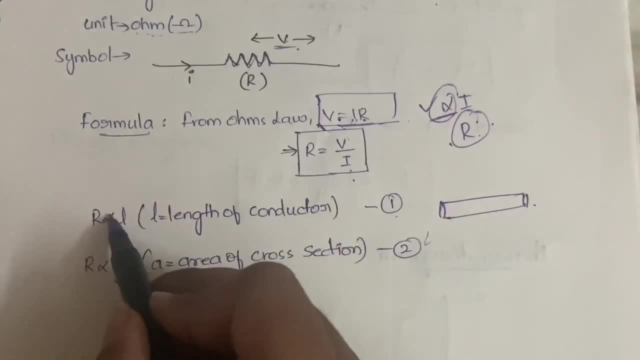 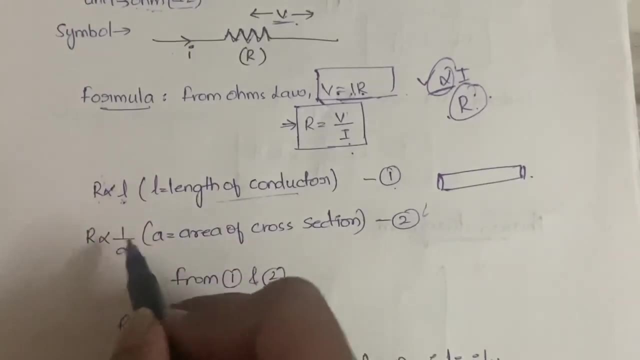 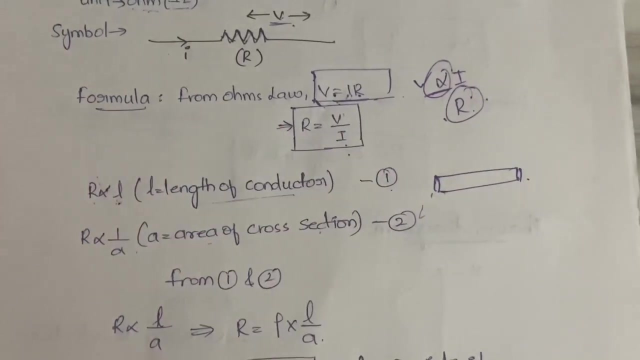 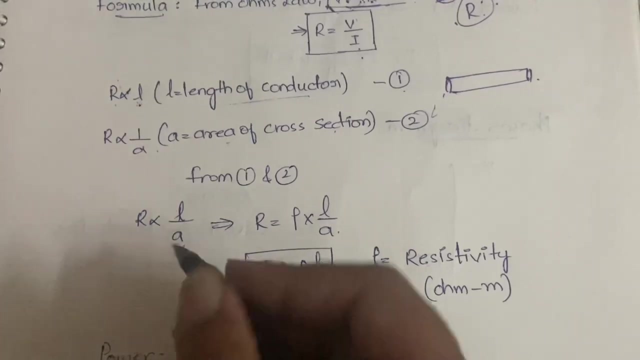 so if you are assuming a conductor, then R is directly proportional to length, length of the conductor. Resistance is directly proportional to the length of the conductor And it is inversely proportional to the area of cross section of the conductor. Got it So from both 1 and 2 equations. what you can say by combining both 1 and 2, you can say that R is directly proportional to L by A Right. So whenever you remove the proportionality, whenever you are making it as is equal to, you will be getting a constant. 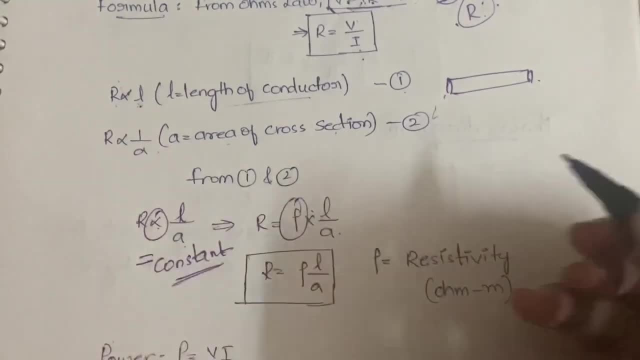 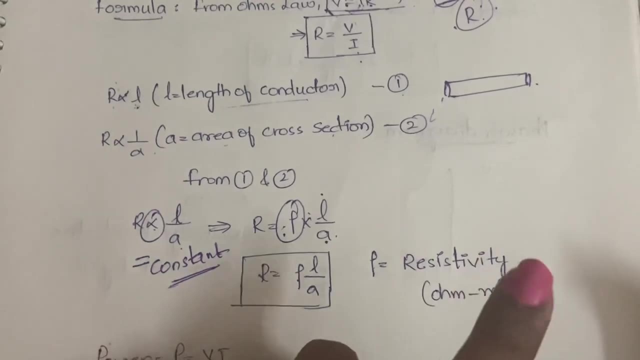 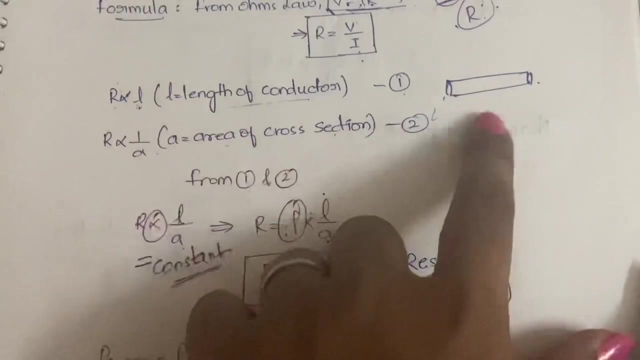 Right. So that constant is nothing but rho here. So R is equal to rho into L by A, where rho is called as the resistivity and the unit of rho is ohm meters. Okay, So R is directly proportional to the length of the conductor and it is inversely proportional to the area of cross section of the conductor. So if you are combining these two equations, you will be getting a. R is directly proportional to L by A And on removing this proportionality you will be getting the constant. That constant is nothing but the. 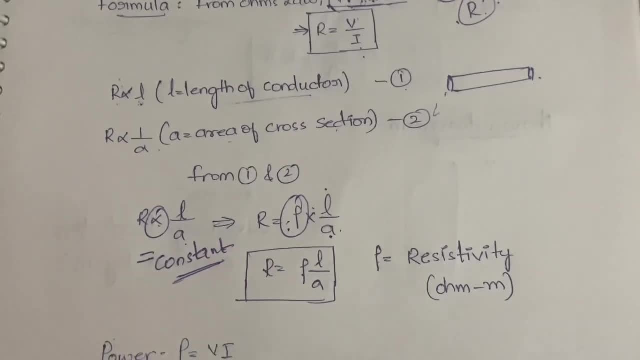 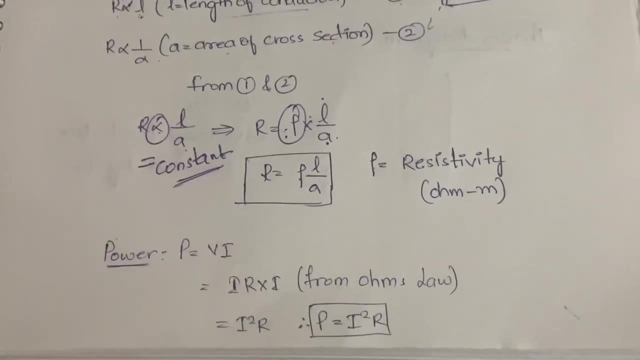 resistivity, okay, and we have another formula also. basically, this formula is to calculate the power. okay, so power formula is v into i in all the three cases: in case of capacitance, in case of inductance also, the formula for power is p is equal to v into i. now, what is v ir? so v is equal. 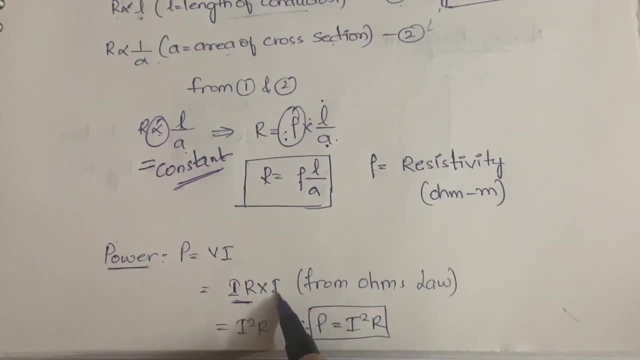 to ir from ohm's law. and what is i current? as it is, you're keeping it ir into i. i square r, p is equal to i square r. so when you're given current and resistance, you can find out power in this way. okay, so for everything, for resistance, for inductance, for capacitance, for everything. 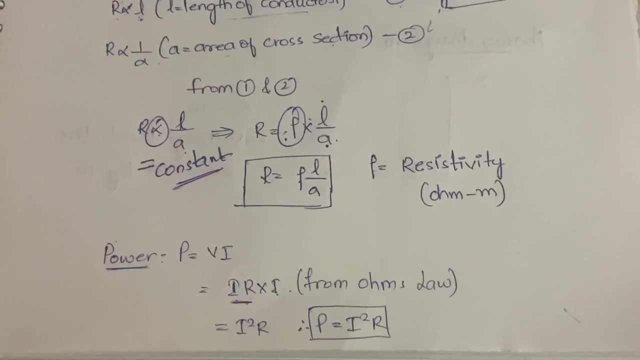 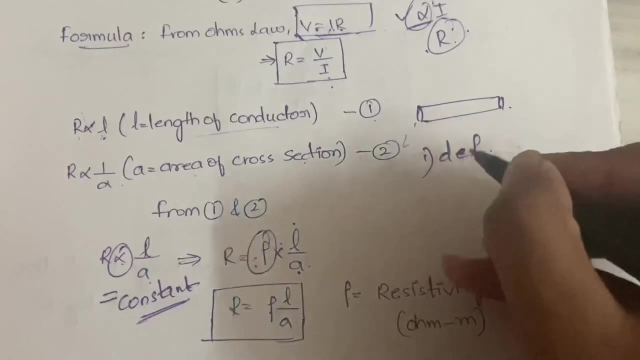 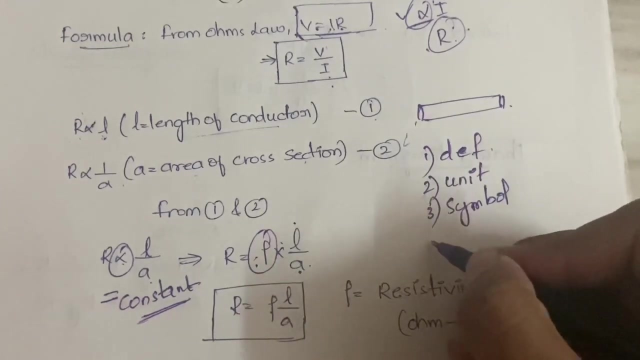 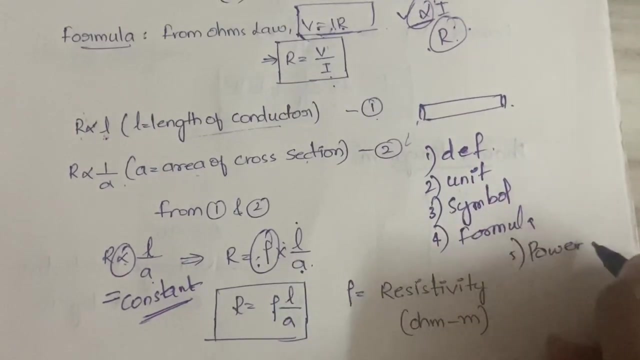 in the exam, if you are asked to explain about the electrical circuit elements, first you have to write the definition, okay. next unit symbol and fourth is formula, fifth is power equation and sixth, phasor diagram. okay, all these six, six things. you have to write for both, for each resistance, inductance and 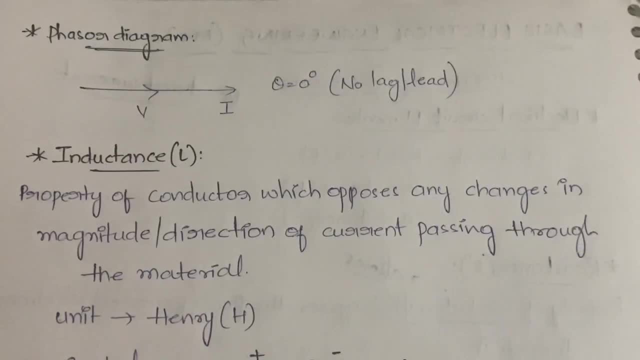 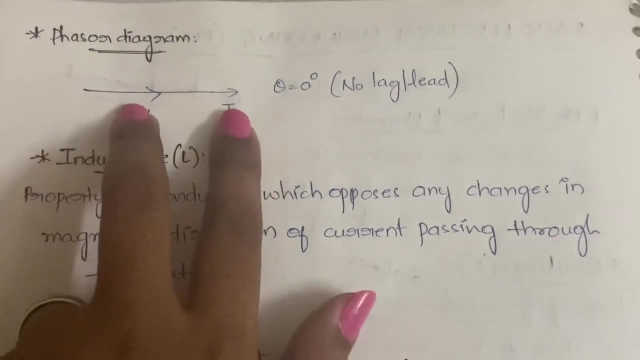 capacitance in the exam, if you are asked this question. okay, next phasor diagram for resistance. so the place was not enough in the previous page. that is why i have drawn it here- see voltage and i. both will overlap with each other. sorry potential difference. and the current. both will overlap. 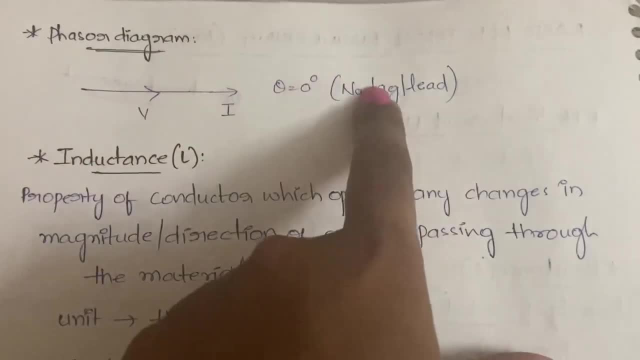 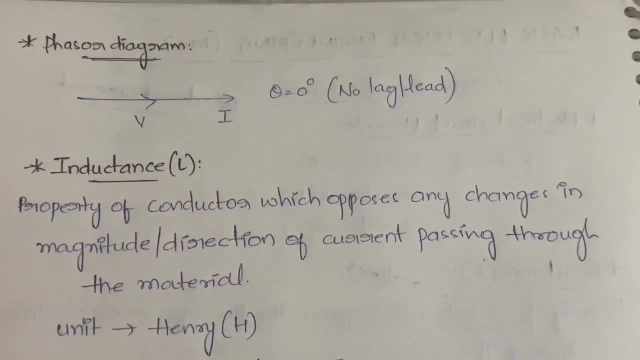 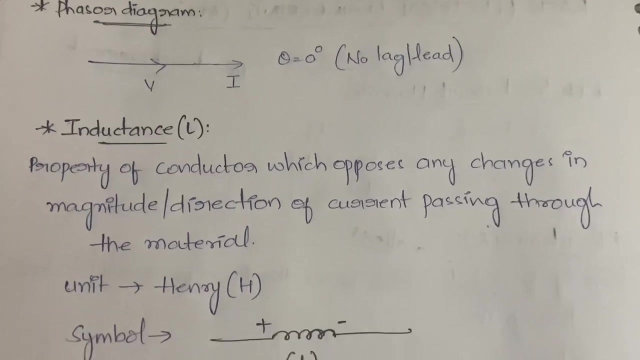 will with each other. okay, no lag or no lead. theta is equal to zero degrees. no lag, what is lag, what is lead? you will understand. next, in the inductance and capacitance, you will understand what do you mean by lag and what do you mean by lead. okay, now, second is second circuit. element is inductance. 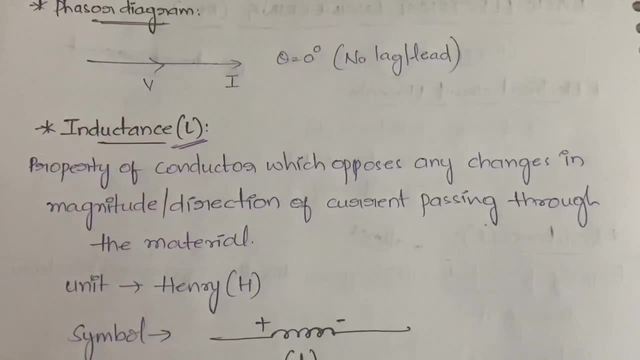 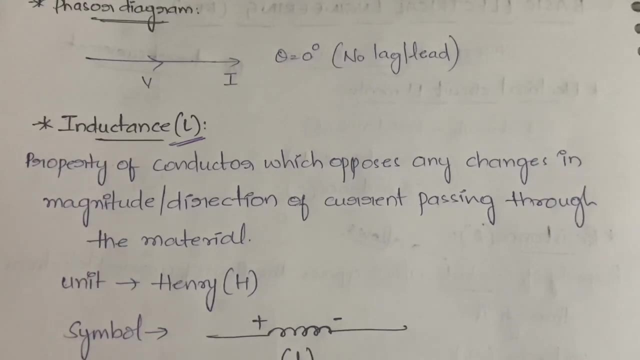 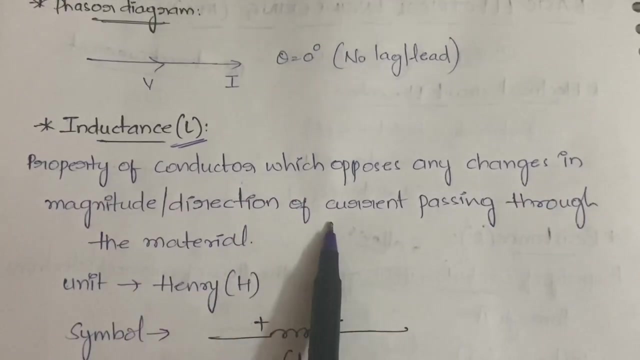 inductance is usually represented with the symbol l. okay, so what do you mean by inductance? the property of the conductor which opposes any change in the magnitude or direction of current passing through the material. don't get confused. see, whenever you are confused with a definition, come from. 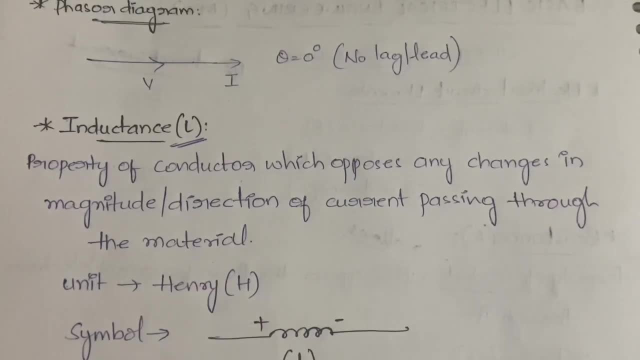 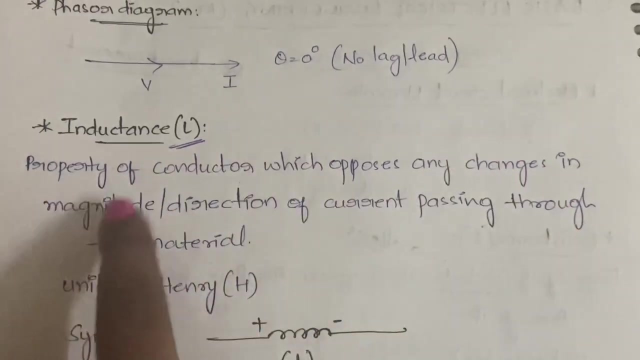 the last come in the reverse direction. if then also if you are not able to understand, then nobody can do anything. so current passing through the material, any changes which are happening to the magnitude or direction is the property of the conductor, which opposes any change in the giant scale. 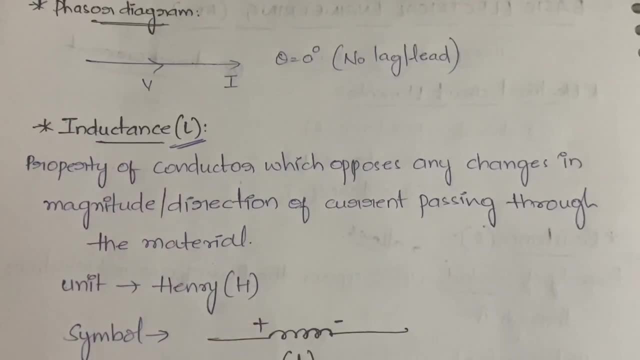 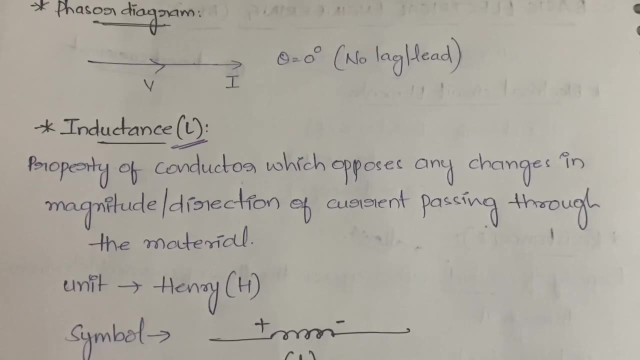 direction of the current passing through the material. see, current is a vector quantity or a scalar quantity. okay, keeping that aside, basically, magnitude or direction in terms of magnitude or in terms of direction. in terms of magnitude, in the sense, suppose, if the value of current is 3 amperes and it has changed to 6 amperes, the value has changed, right this? 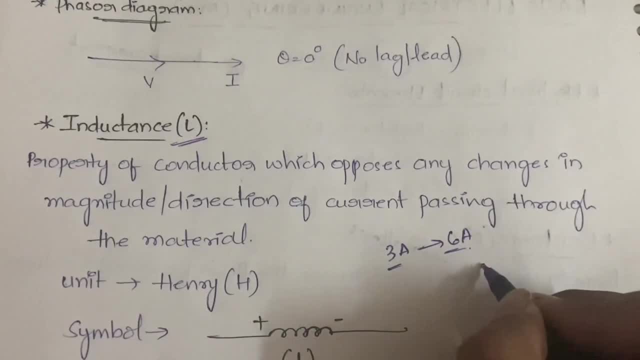 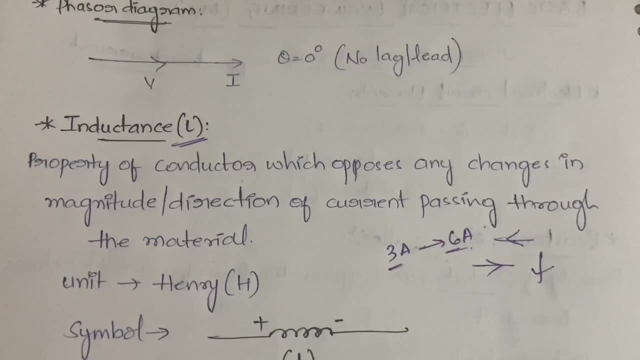 is change in magnitude, change in direction is nothing. but if the current is flowing in this direction, suddenly it got changed to in this direction or it got changed to this direction, whichever. so if the direction or the magnitude of current is changing, then that changes should not happen. who is responsible for that? who will take care of that? conductor? 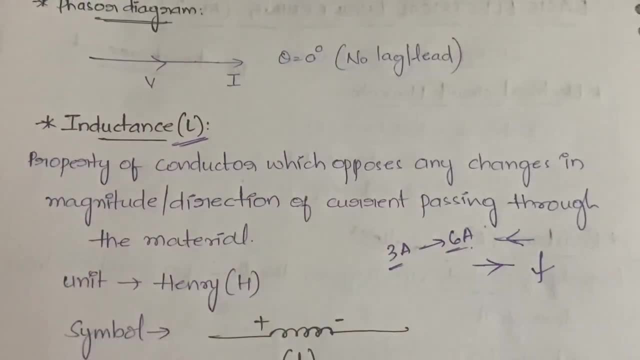 the conductor will oppose. i mean sorry, sorry, sorry, inductance. so inductance is a property which will oppose the changes which are happening in the conductor, changes related to what current. it could be in the magnitude wise, or it could be in direction wise. so these 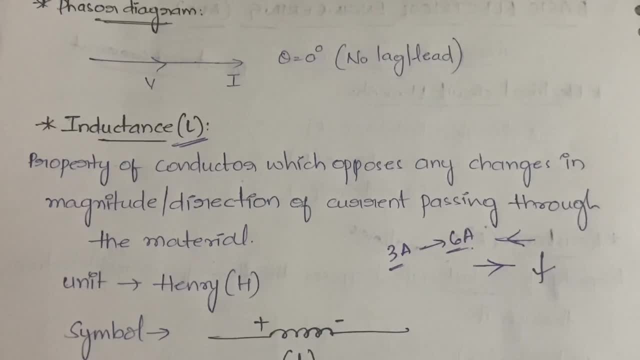 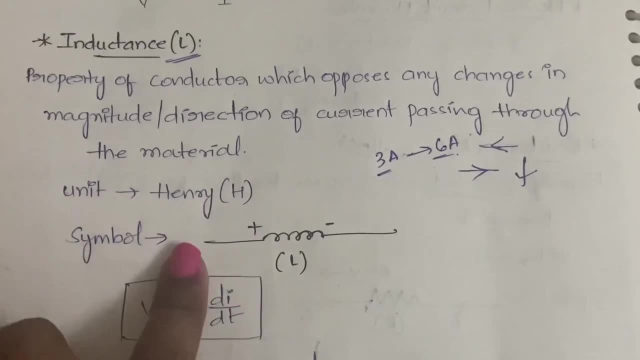 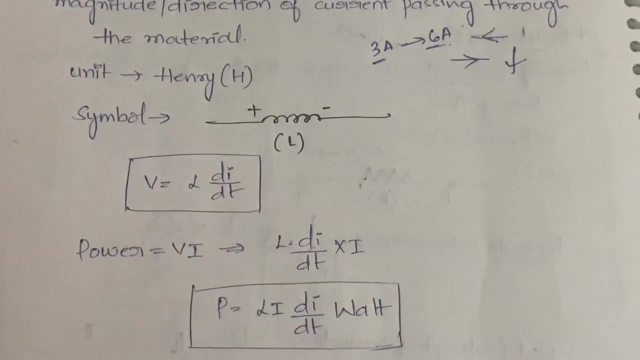 two changes will be opposed with the help of the inductance property. okay, done. next, what is the unit, henry? it is denoted by h and symbol is like this: coil. okay, next, v is equal to l into di by dt. this is the formula we have. so for inductance, next power, power. 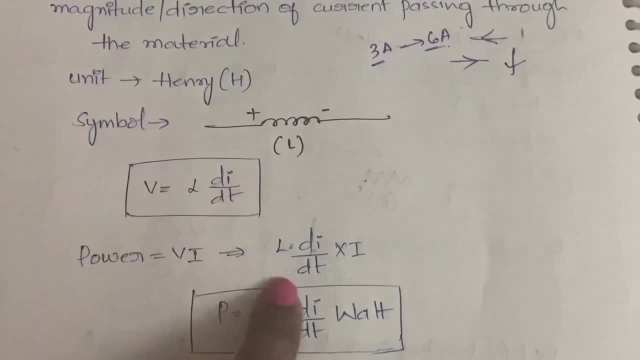 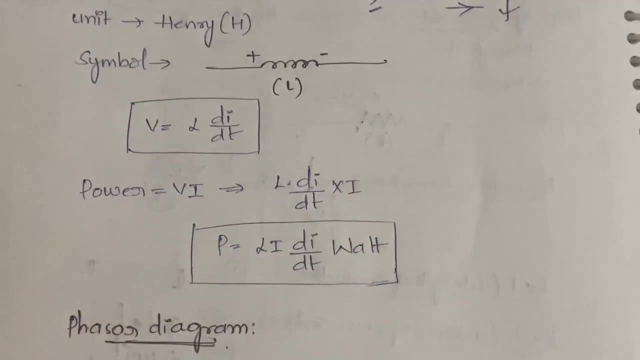 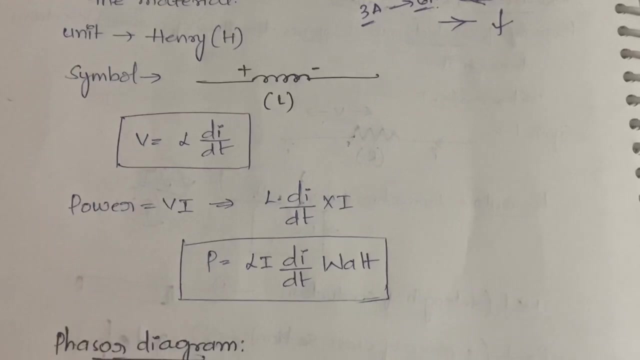 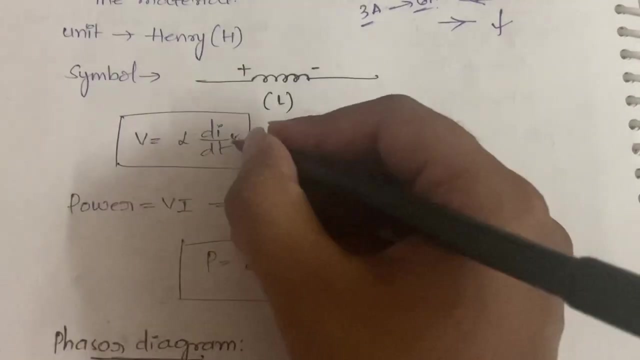 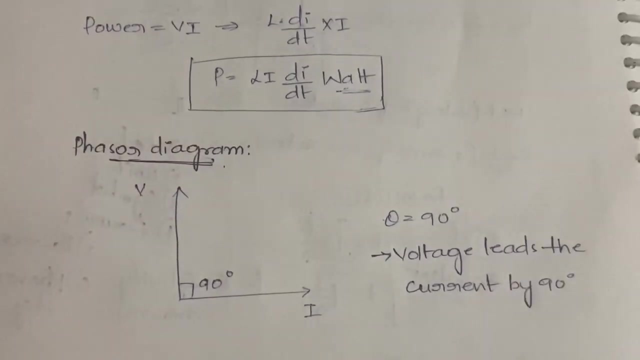 is equal to vi. you already know that what is v? v is equal to l into di by dt. this is the formula we have. so for inductance, next, power, power is equal to vi. you already know that what is v here? l into di by dt into i. so p is equal to. you are bringing this i over the side li di by dt. di by dt is nothing but the change in current. so here, as we said, changes in the current, so that change in current is di by dt. okay, and the unit of current power is what. so we have written it as what. and here also you can write v like voltage. but if i write v again you will get confused. right again, one more v. so i have not written. now let us go to the phasor diagram. so in phasor diagram, 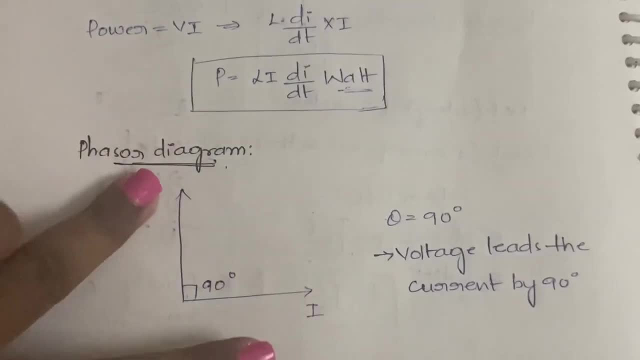 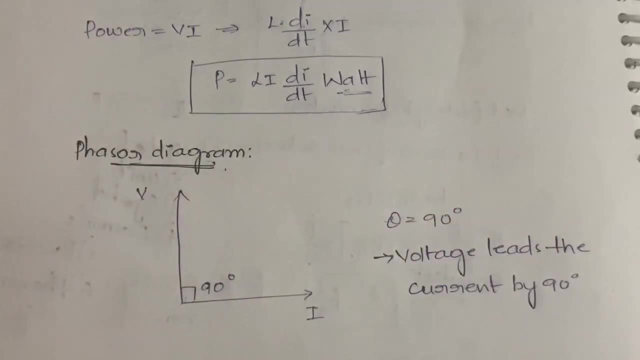 this is the potential difference and this is the current. okay, potential difference, current. now the angle between the current and the potential difference is 90 degrees. so we have written: theta is equal to 90 degrees. now, which is leading, which is lagging? leading in a sense, which is above, which is up. see, leading means what? lagging? 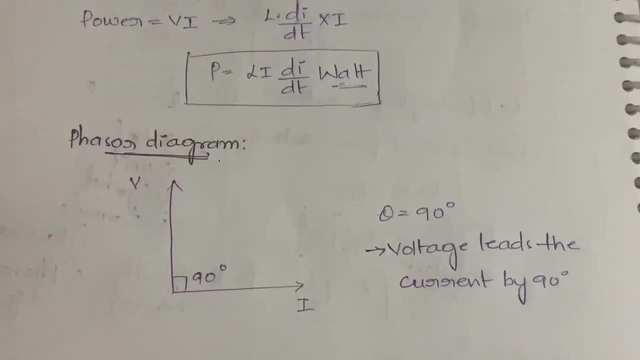 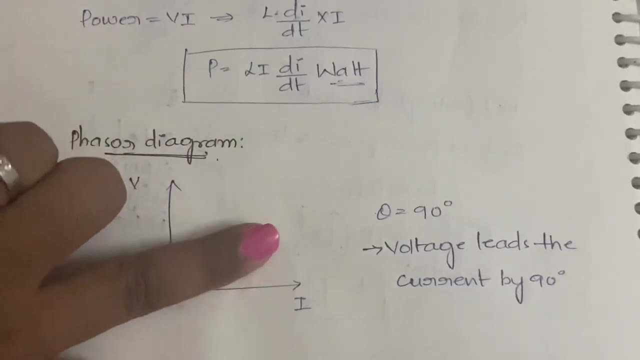 means what? it has a lot, of, lot of physics theory involved in it, but for time being i'm telling you which is on the top. voltage is on the top right, so volt from here to here 90 degrees, and which is the top of 90 degrees voltage. so that is why voltage is leading the current by 90 degrees. 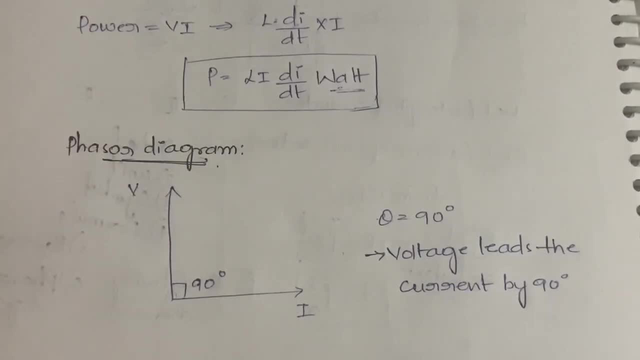 got it, voltage is leading the current by 90 degrees. this is about the inductance phasor diagram. simple inductance is nothing, but it is a property of the conductor which will oppose the changes which are happening to the magnitude or direction of the current in the conductor. 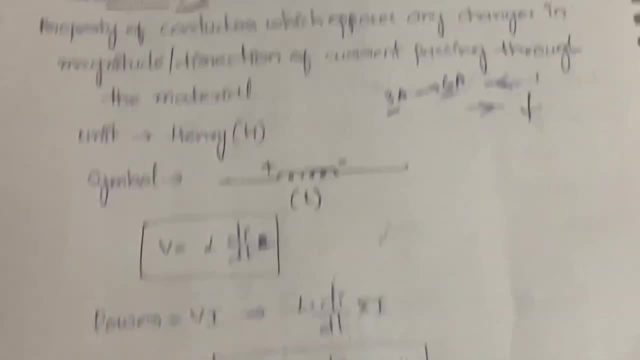 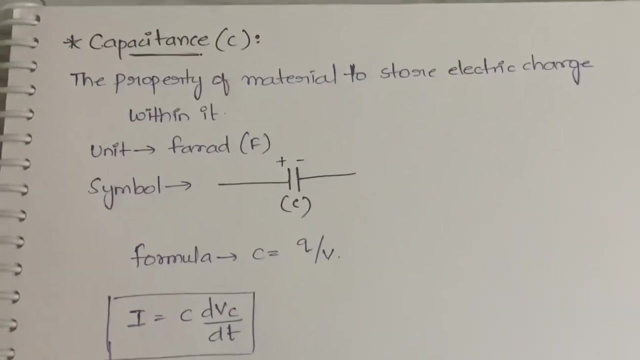 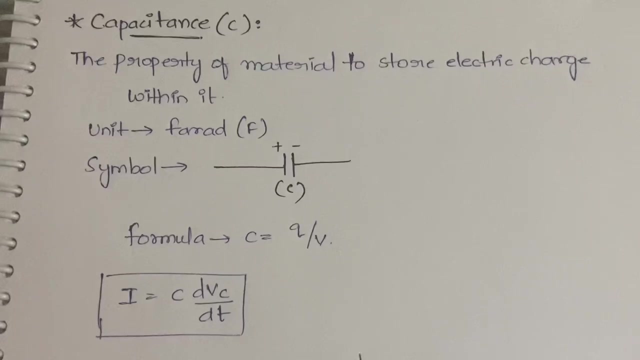 got it, and unit is henry and the symbol is this coil kind of thing and the formula for power and phasor diagram. all now let us move to the next thing, that is, the capacitance. so capacitance, also simple. let me check if i have missed any points in inductance. no, now let us check capacitance. 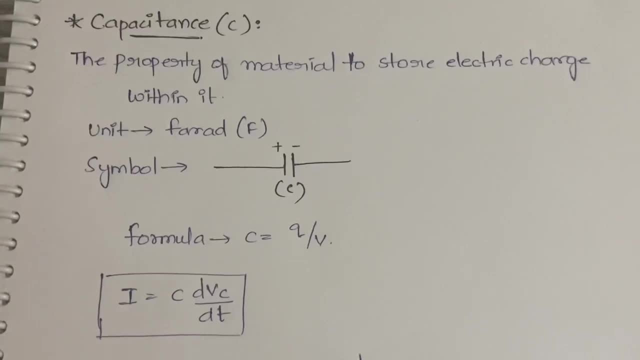 it is the property of material to store electric charge within it. it's simple: it is the property of the material to store the electric charge within it and the unit of capacitance is farad. f a, r a d farad, it is denoted by f. okay, and 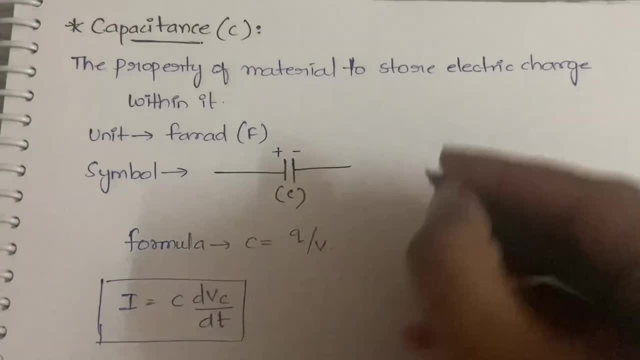 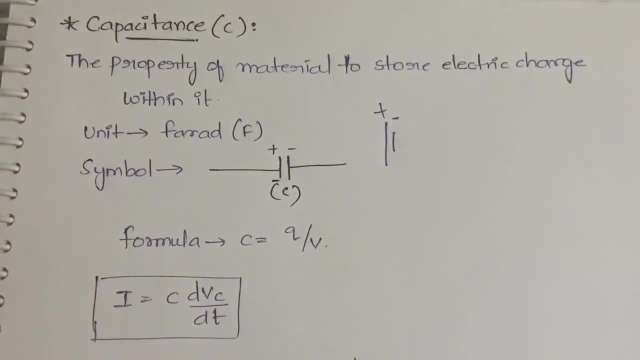 the symbol is this one see, don't get confused with the symbol of battery. battery will have one line big and one line small. this is battery. but capacitance- two lines, both positive and negative- terminals will be equal in length. okay, that is the difference between the capacitor. 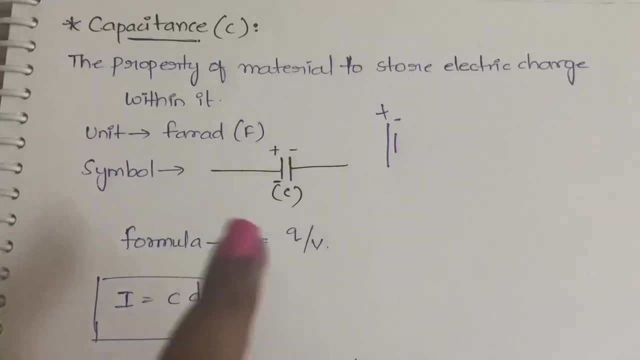 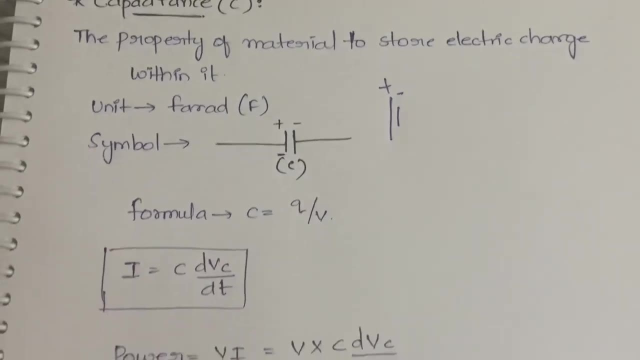 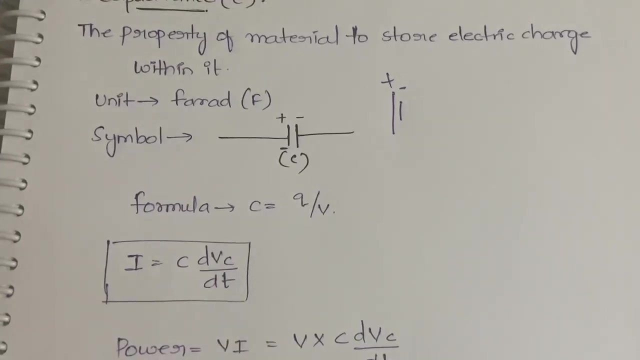 and the battery. okay, don't get confused. so this is the uh. this is the symbol of capacitance next to formula. c is equal to q by v. or we have other formula like i is equal to c, v, c, d, v, c by dt or c. if you're getting confused between inductance and capacitance, simple, their voltage will play.